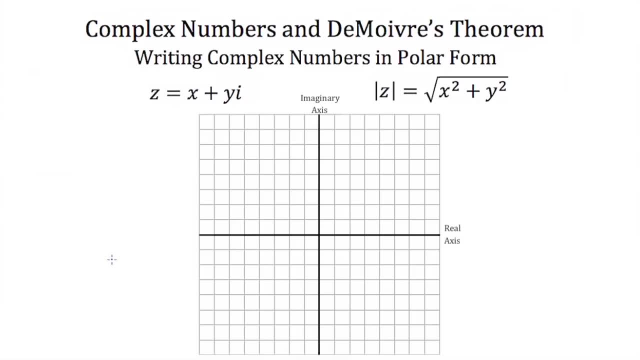 Now, typically if we want to plot a complex number, we plot it on a rectangular axis where the x-axis or the horizontal axis is the real axis and then the y-axis or the vertical axis is our imaginary axis. So if i have a plus b? i or 5 plus 7i, then my imaginary number z, instead of saying it's a plus. 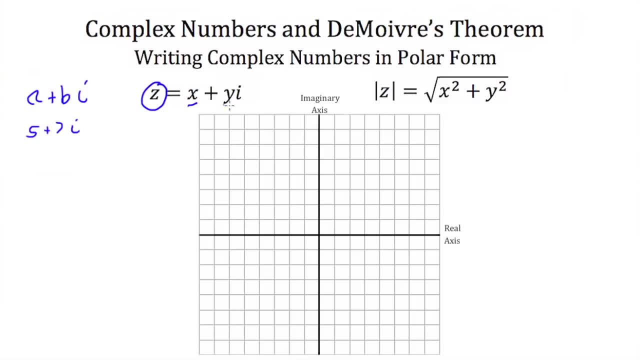 b, i. i could say that it's x plus y, i, and in this case x. or my real part is 5 and my imaginary part, y, is 7.. Or you can think 7i, and if i wanted to plot this i would go along the real axis. 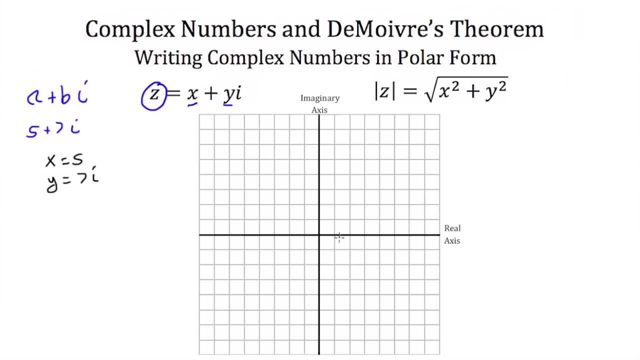 my real part, or in this case, 5 units, and then i would go up along the imaginary direction or the imaginary axis, my y part, or 7, to this point right here, this is the point z. Now, when you take the absolute value of an imaginary number or a complex number, 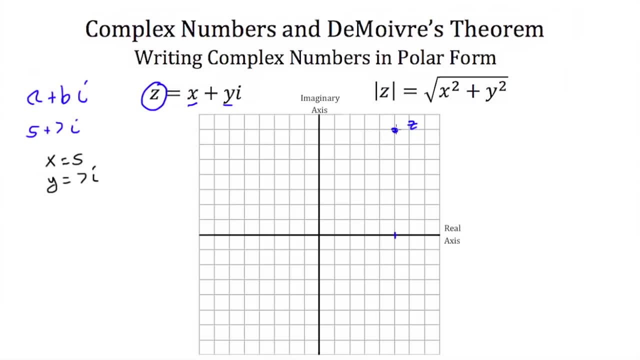 remember that the absolute value is the distance that point is from the origin. If we were taking the absolute value of 5, well that's just 5, because it's 5 units away from our origin. If we want to find the absolute value of a complex number, though, 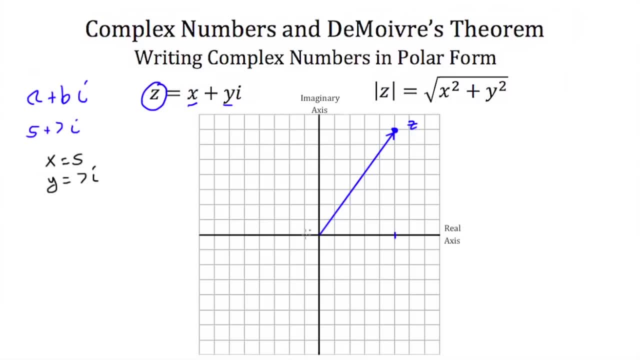 We would want this distance. This distance is the absolute value of z. Now, if i want to find the absolute value of z, i can think of this kind of like a triangle, And then i can use the distance formula, or i can use Pythagorean's theorem, because this: 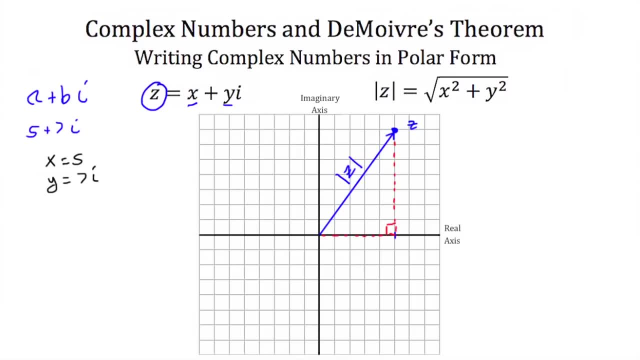 is a right triangle. so I take my X part and I square it, and I add that to my imaginary part, or my Y part, which is also squared, and I take the square root. this is the square root of 25 plus 49, or the square root of 74, which, if you're curious, is about 8.6. 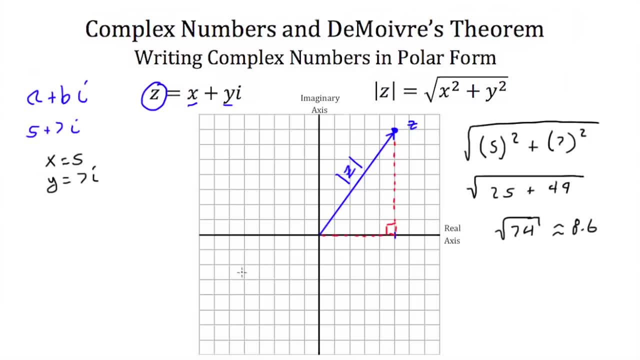 well, you may notice that finding the absolute value of our complex number is a lot like converting our complex number into a polar coordinate system. if I said this absolute value of Z, that would also be distance R, and then all I would need is a theta value. remember, when you convert from rectangular. 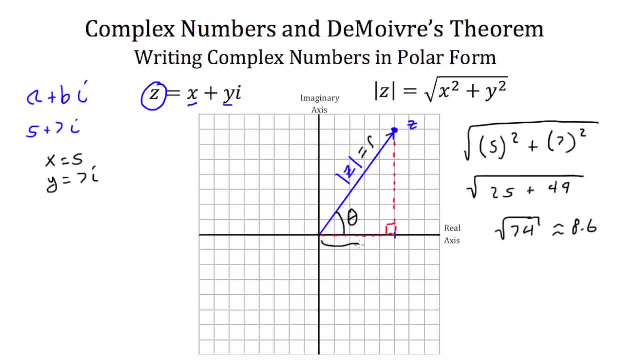 to polar coordinates. this X value here, this is always equal to R times the cosine of theta, our hypotenuse length times the cosine of this angle. and then our Y value: this is always equal to R times the sine of theta. but remember you that we're going in the imaginary axis. this is not the Y axis, this is the 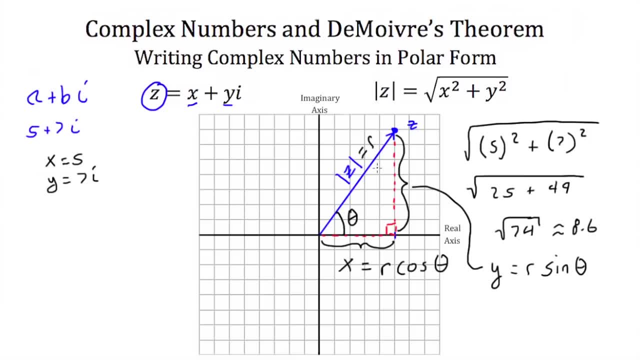 imaginary axis. so even though I'm calling this Y, this is really R sine theta times I times the square root of negative 1. so if I wanted to, I could take this form and I can say: Z is equal to R cosine theta plus R sine theta times I. this is X, this is Y and if I factor out an R, I'll get Z is. 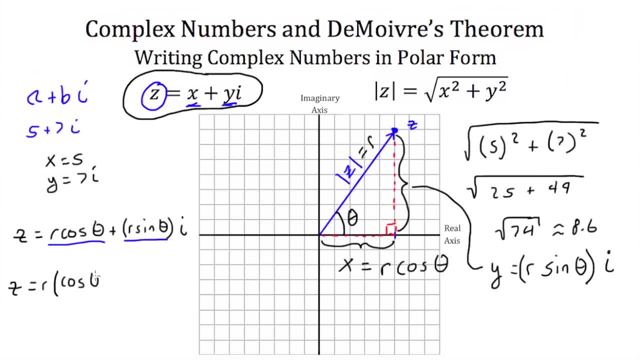 equal to R times the cosine of theta plus I, sine theta. well, this is how you write complex numbers in polar form. if I wanted to find theta, I could use the tangent function, because the tangent is just the opposite side length over the adjacent side length. so the tangent of theta is equal to Y over X. our y is 7 and our X is 5, so the 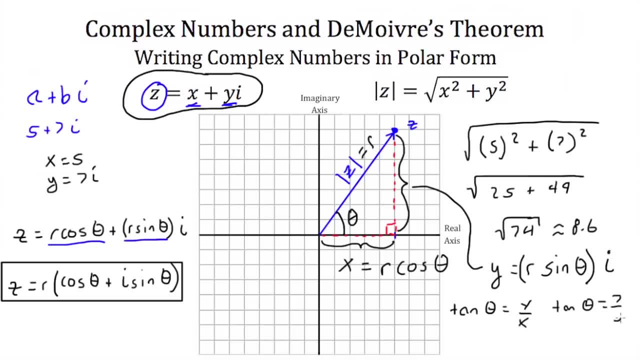 tangent of theta is 7 over 5. put that into your calculator and find that theta is about 54.5 degrees. So if Z is 5 plus 7i, I could write that as the square root of 74, because that's my R value times the. 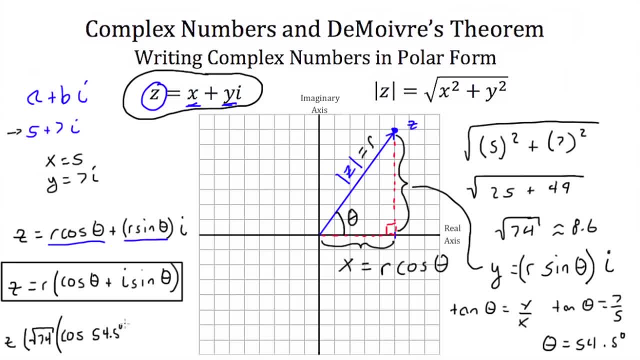 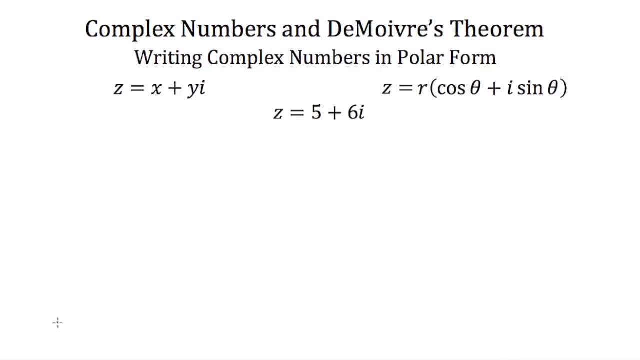 cosine of 54 degrees or 54.5 degrees, plus I times the sine of 54.5 degrees. So let's try this again. Let's write a complex number in polar form. Remember: normally it's Z is equal to X plus YI. When we want to make it, Z is equal to R. 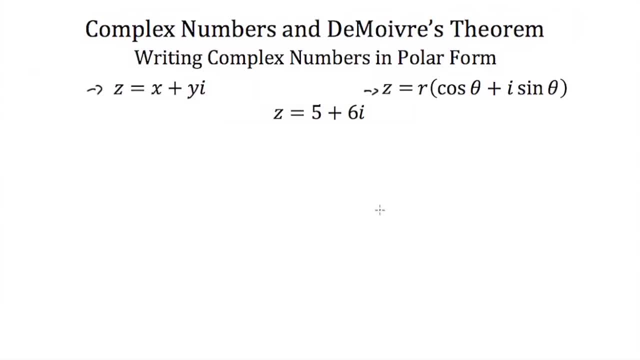 plus YI Times the cosine of theta, plus I times the sine of theta. So let's convert: Z is equal to 5 plus 6i- into polar form. Now it usually helps to first draw a triangle. The bottom of my triangle follows the X, or you can think of the. 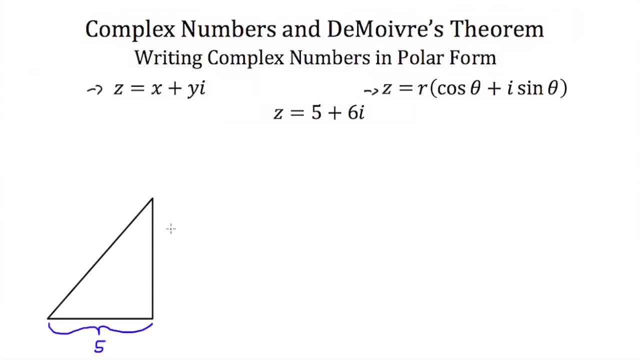 real axis and this length here is 5.. This side of my triangle is 5, and this side of my triangle follows the imaginary axis, or you can think of that as the Y axis, and then this length is 6.. So if I want to write this in polar form, I'm going to 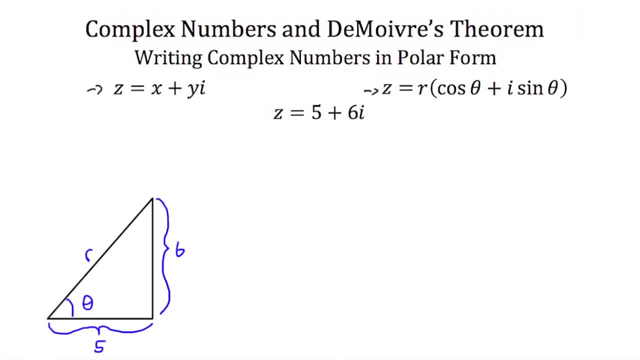 need an R value and I'm going to need a theta value. Well, to find my R, I'm going to take the absolute value of this number. So I'll have the square root of 5 squared plus 6 squared. This is the square root of 25 plus 36, or you can think of that as the square root of 61.. 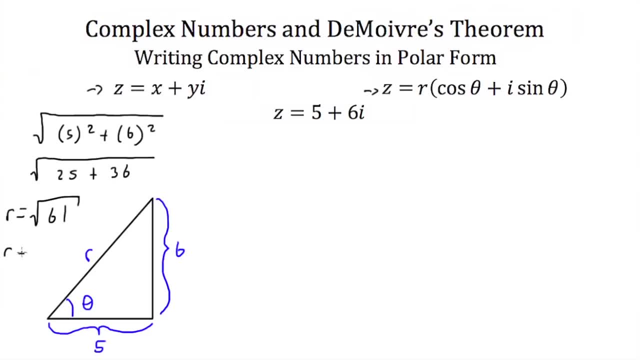 So this is our R value. If you're curious, this is about 7.8.. So we have our R value and we're going to need our theta value. So I'm going to use the tangent function to find that, Remember, the tangent of theta is equal to 6.. 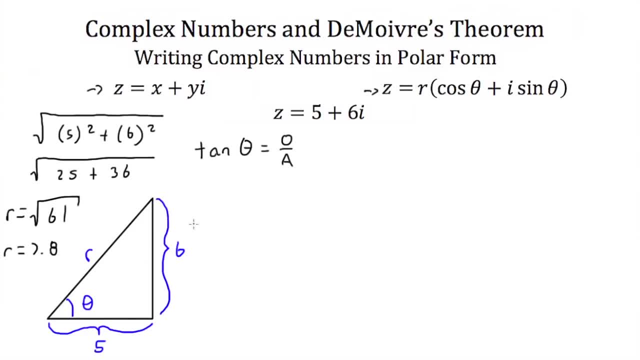 It is equal to opposite over adjacent. So the tangent of this theta- the opposite side length- is 6 and the adjacent side length is 5.. So the tangent of theta is equal to 6 over 5 and if you plug that into your calculator you'll find that theta is about 50 degrees. 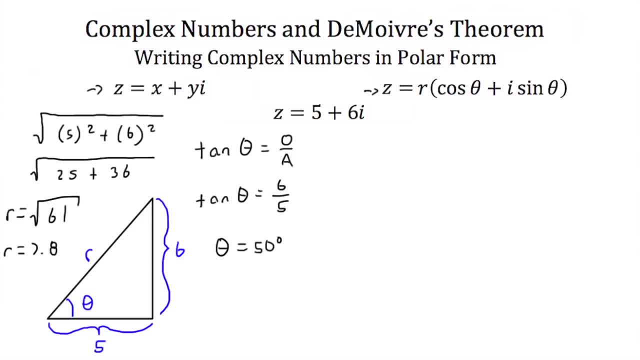 So I have everything I need. So I'm going to write this in polar form. So Z is equal to our R value, which is the square root of 61 times the cosine of 50 degrees, plus I times the sine of 50 degrees. 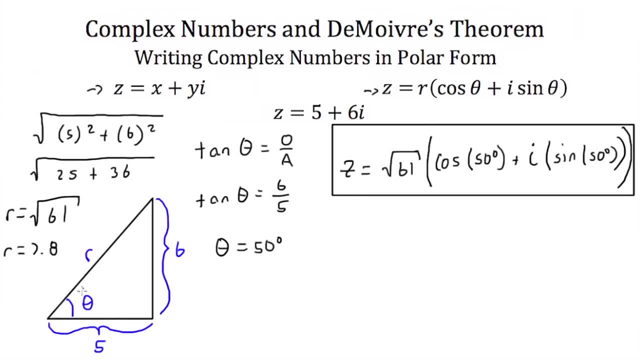 Now, if you don't want to remember this formula, you can always remember the conversions from regular to polar coordinates. You can remember: x is equal to R cosine theta and y is equal to R sine theta, And then you can plug these values in for x and y and you'll end up with the same number. 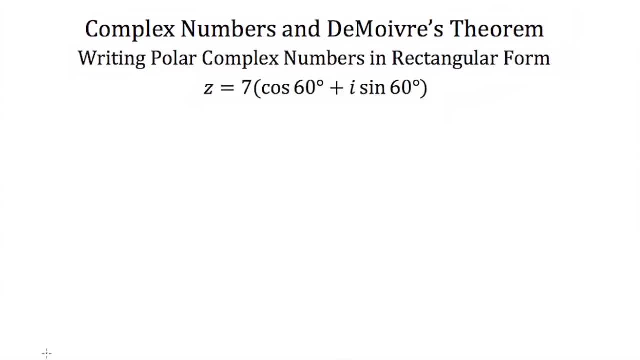 So now let's try going the other way. Here we have a complex number written in polar form. Let's get it out of the way. Okay, Here we add in our 0 value to our equation. So our 0 value equals 1 over 2. That will be 1 over 6.. 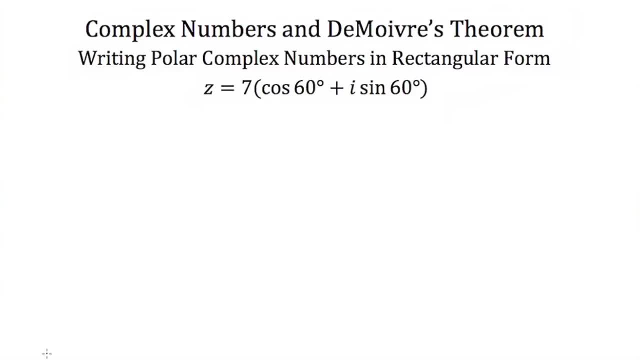 form, and we want to write it in the rectangular form that we're used to Here. z is equal to 7 times the cosine of 60 degrees, plus i times the sine of 60 degrees. Well, usually I like to start by drawing a triangle. It doesn't have to be to scale, it just has to help me see what's going on. 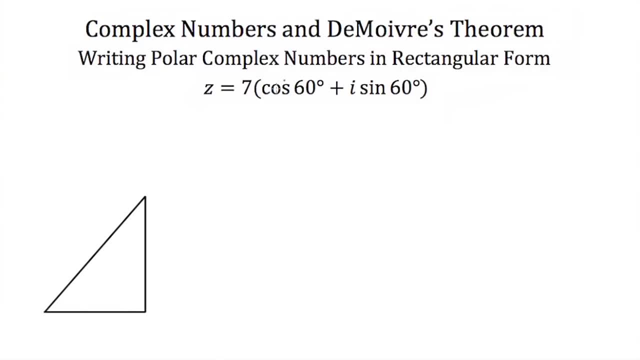 Now, when we're written in complex or polar complex form, z is equal to r times the cosine of theta, plus i times the sine of theta. This distance is r and this distance is theta. This distance is y and this distance is x. Well, I have my r value. r is 7, so this is 7.. 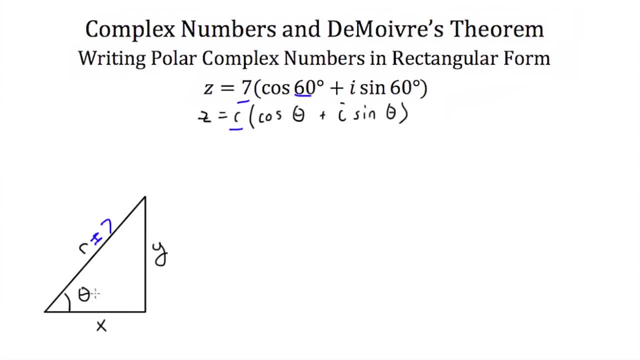 And I have my theta value that's 60, so this is 60 degrees. Now, using the sine function, remember that sine of our angle is equal to the opposite. over the hypotenuse, This is a right triangle. so the sine of theta, which is 60 degrees, is equal to the opposite side, which is y. 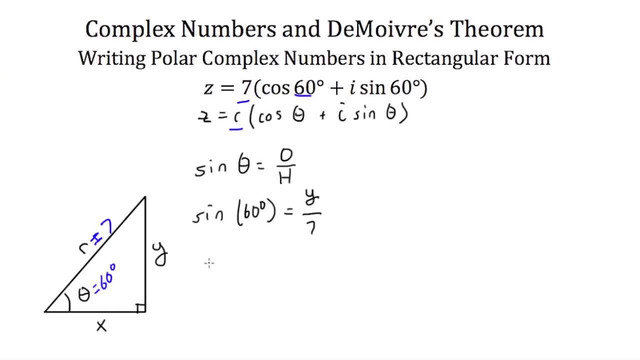 over the hypotenuse, which is 7.. So y is equal to 7, sine 60, and this is equal to approximately 6.06.. For my x value- well I know- the cosine of theta is equal to the adjacent side length. 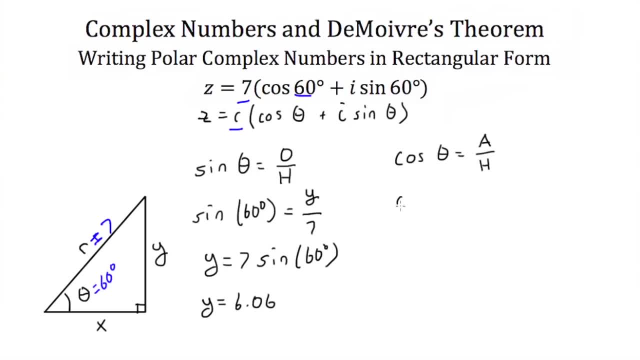 over the hypotenuse. So the cosine of 60 degrees is equal to x over 7.. So x is equal to 7 times the cosine of 60 degrees And we'll find that x is equal to 3.5.. So I have my x and my y value. but remember, this isn't a normal x and y. this is actually the real. 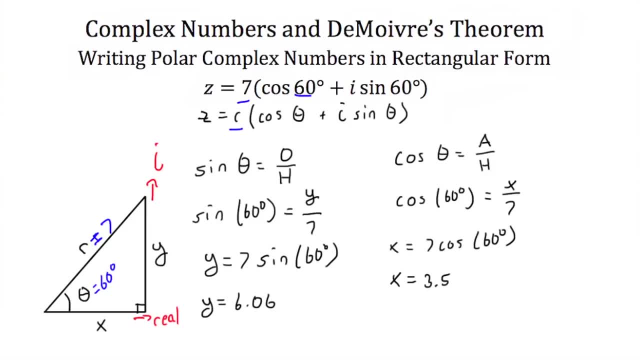 and the imaginary axis. So that means z is equal to 3.5 plus 6.06 i, Because remember complex numbers in rectangular form look like z and y is equal to x plus y, i or a plus b, i. here our x is 3.5 or a is 3.5 and our y or b value is 6.06. 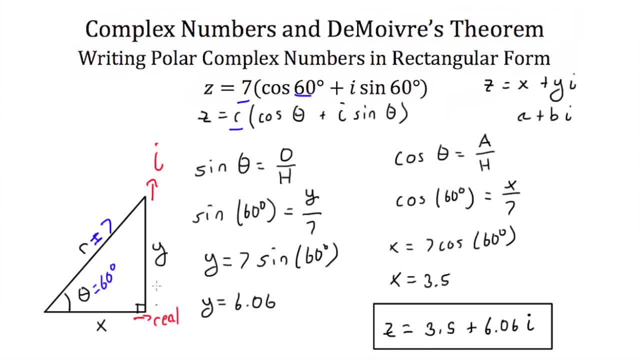 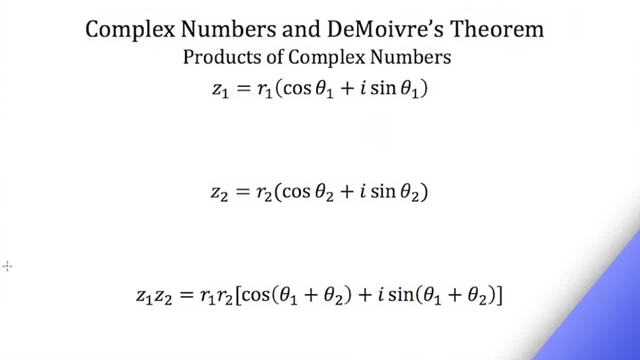 just don't forget to include our i for the b or the y value. so now let's talk about taking the product of complex numbers. normally, if we had a plus b i and we multiplied it by c plus d i, we would have to foil this out. well, when our complex numbers 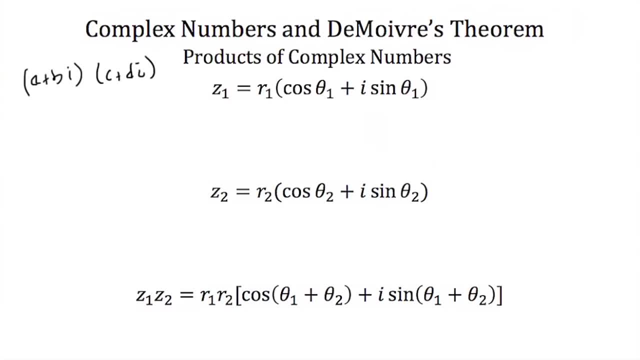 are written in polar form. say, complex number one has a rf of a plus b i and rf of a minus b i value of 1 and a theta value of 1. so it's written in this form. And our second complex number, Z2, that has a different R, so we'll call it R2 and theta 2.. So if we 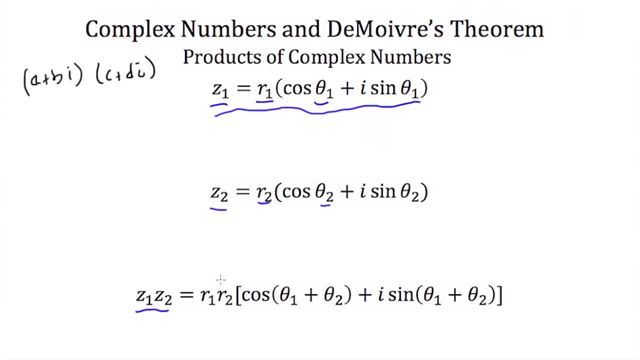 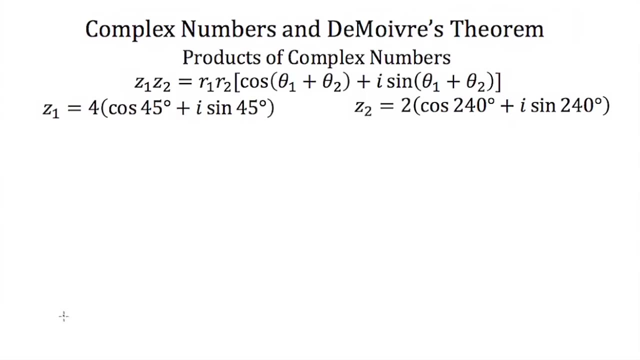 want to multiply Z1 and Z2. we just multiply their R values and then inside the cosine we add the theta values and then inside the sine we add the theta values. So let's multiply these two complex numbers. in polar form, Z1 is equal to 4. 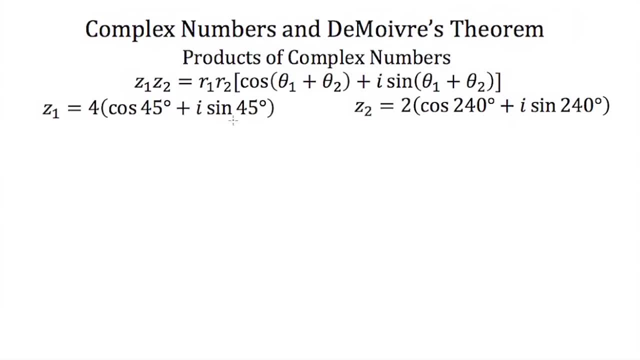 times the cosine of 45, plus I times the sine of 45.. Z2 is equal to 2 times the cosine of 240 degrees, plus I times the sine of 240 degrees. We're multiplying. So Z1 times Z2, I'm going to use my formula- is R1 times R2.. 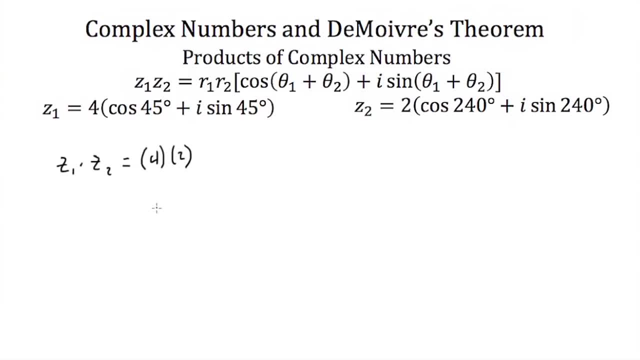 So 4, times 2, and then times the cosine. Now I add my angles, so 45 plus 240.. And then plus i times the sine of 45 plus 240.. So z1 times z2 is 4 times 2, which is 8, times the cosine of 45 plus 240, is the cosine of 285 plus i times the sine of 240.. 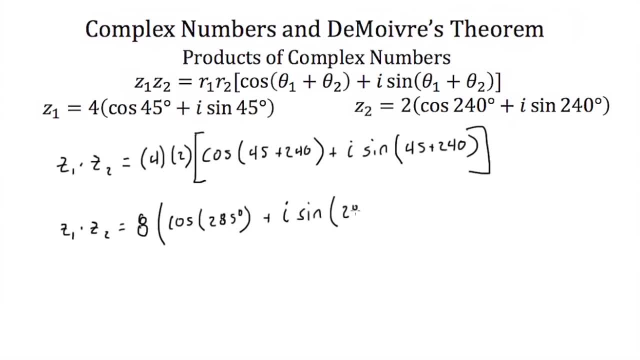 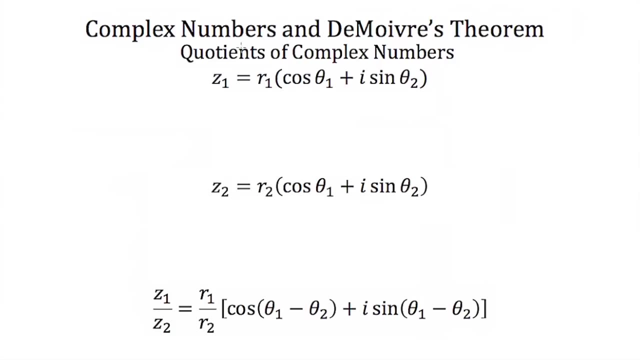 The sine of 45 plus 240, 285.. And that's how you multiply two complex numbers written in polar form. So now let's talk about dividing complex numbers or the quotients of complex numbers. Well, this is just like multiplying. 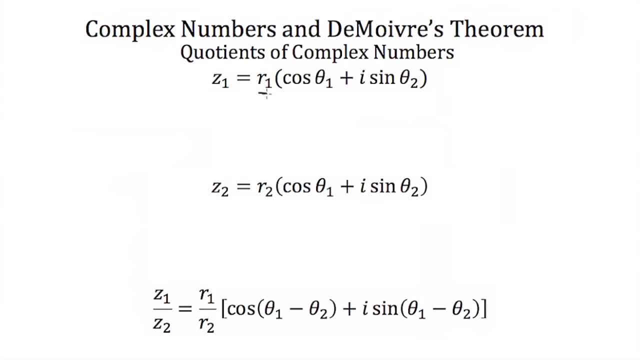 Instead of multiplying our r values, we're going to divide them, And instead of adding our theta values from our two numbers, we're going to subtract them. So if we're dividing z1 by z2, then you're dividing r1 by r2.. 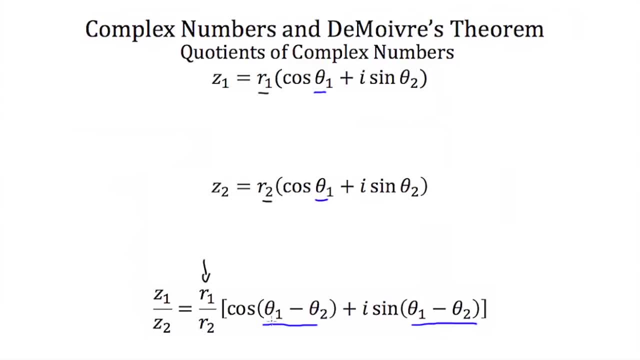 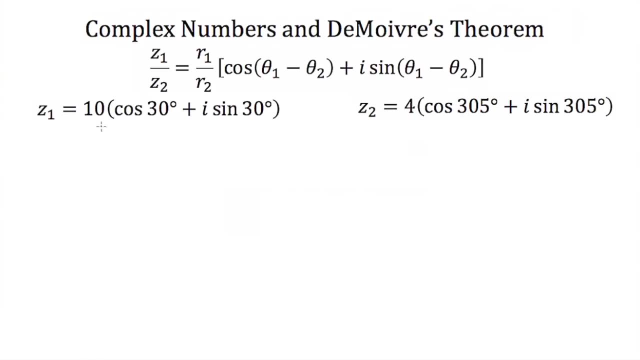 And you're subtracting theta2 from theta1.. So let's practice this. We have: z1 is equal to 10 times the cosine of 30, plus i times the sine of 30.. And z2 is equal to 4 times the cosine of 305 degrees. 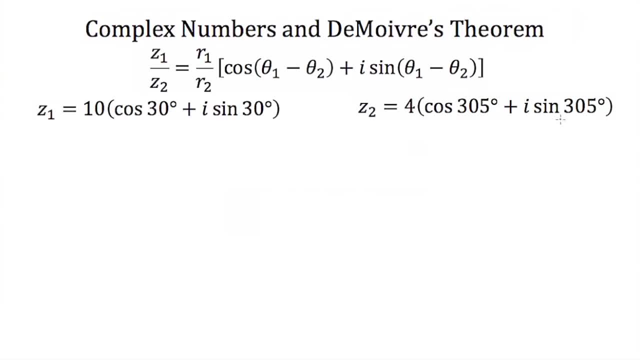 plus i times the sine of 305 degrees. z1 divided by z2,, that's equal to r1 divided by r2, so 10 divided by 4.. And that's multiplied by the cosine of 30 minus 305, plus i times. 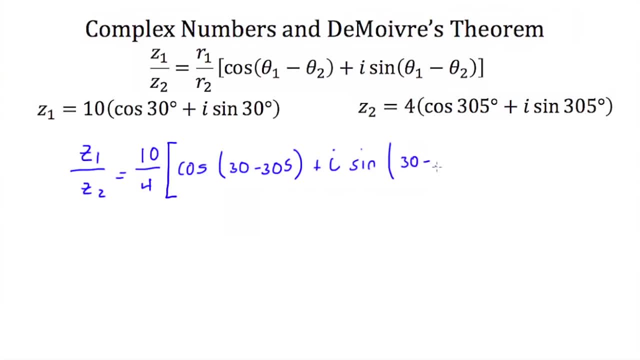 The sine of 30 minus 305.. So Z1 divided by Z2.. 10 over 4, you can think of that as 5 over 2.. That's multiplied by the cosine of now, 30 minus 305, is a negative 275 degrees. 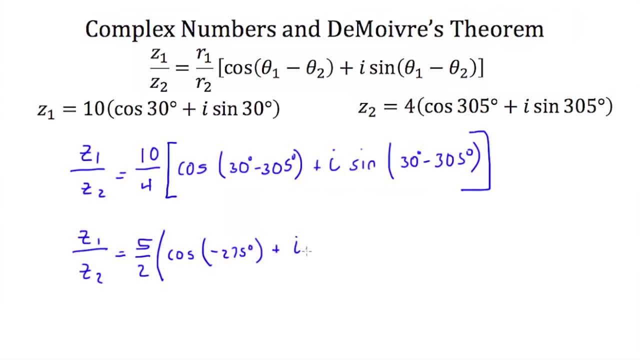 Plus, I times the sine of negative 275 degrees. Now this is an acceptable solution, except I don't usually like to have negative angles. If I start here and I go in a clockwise direction or a negative direction around to 275, I can find a positive angle by going the other direction. 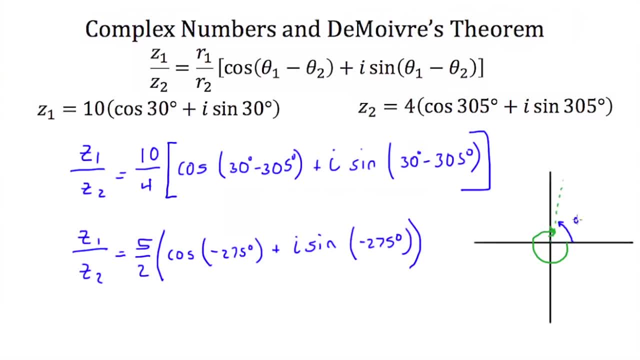 If this is 275, then this is 85. So I'm going to write this as Z1 divided by Z2. And that's equal to 5 over 2 times the cosine of 85 degrees, Plus I times the sine of 85 degrees. 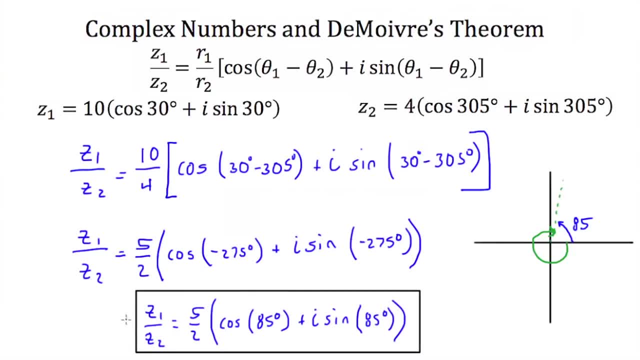 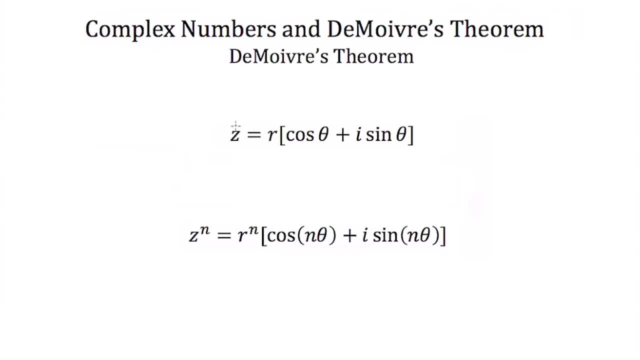 And that would be our solution. So now let's talk about De Morey's theorem. If I have a complex number written in polar form, Z is equal to R times the cosine of theta, plus I times the sine of theta, And I want to raise Z to some power N. 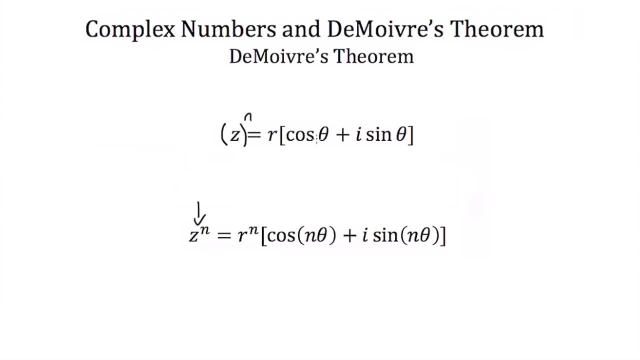 Then, instead of multiplying Z times cosine theta plus, I times the sine of theta by itself. over and over again, I can use De Morey's theorem And that tells us that our complex number raised to the N power, well, that's the same as R to the N power. 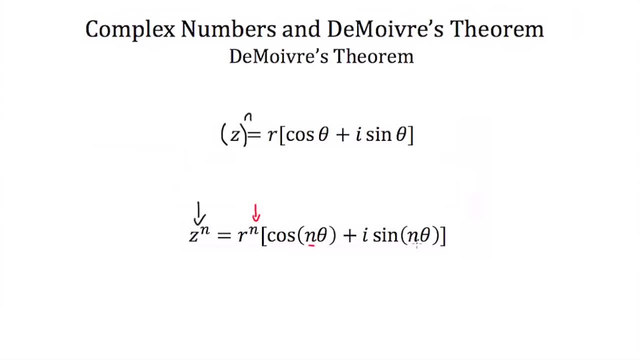 And then the N comes inside our cosine and our sine and we just multiply our angle by N, So it's the cosine of N times theta, plus I Times the sine of N times theta. So again, let's practice this. Here's De Morey's theorem. 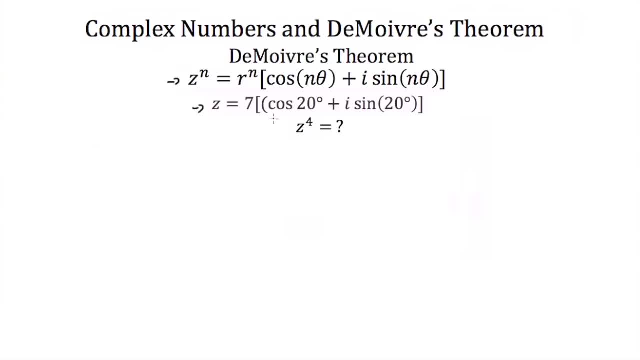 Here's Z. It's equal to 7 times the cosine of 20 degrees, plus I times the sine of 20 degrees. And we want to find Z raised to the fourth power. Well, Z to the fourth power is equal to R to the fourth power. 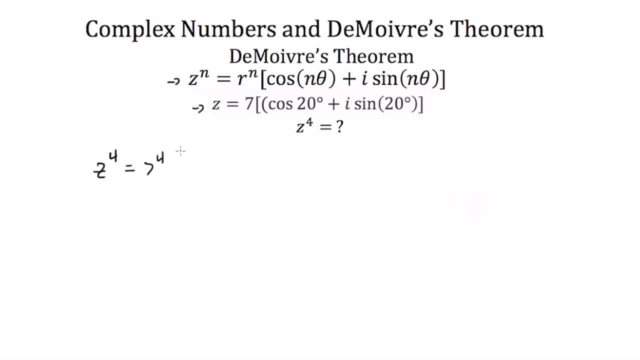 So 7.. Z to the fourth power is equal to 7 to the fourth power times the cosine of N times theta, So 4 times 20 degrees. plus I times the sine of 4 times 20 degrees, So Z to the fourth power is equal to 7 to the fourth power, which is 2,401.. 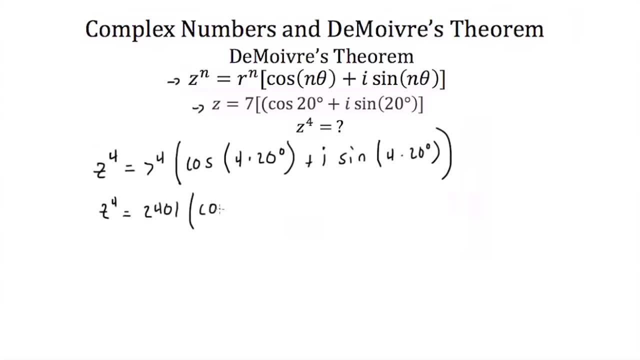 And that's multiplied by the cosine of 4 times 20 degrees or 80 degrees. plus I times the sine of 4 times 20 degrees or 80 degrees, And that would be our solution. So now let's talk about finding the square root of a complex number. 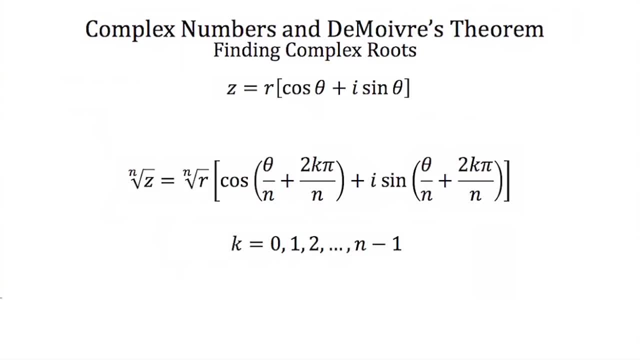 Or at least a complex number written in polar form. Now remember, if I take the square root or the second root of some number, say 4,, I always end up with two solutions, because this can be plus or minus 2.. 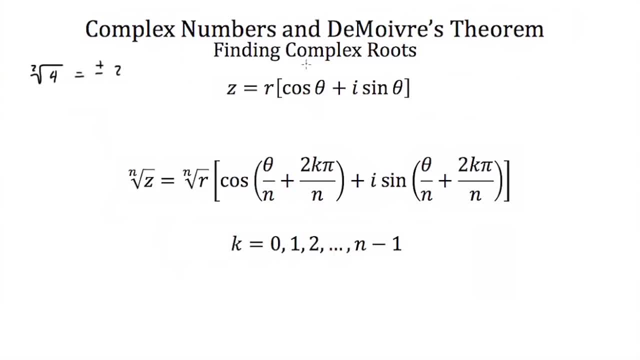 Well, when we find a complex root, if we have the nth root, we have N possible solutions. So if I'm taking the fourth root of Z, I'm going to have four solutions. If I'm taking the square root, I'm going to have two solutions. 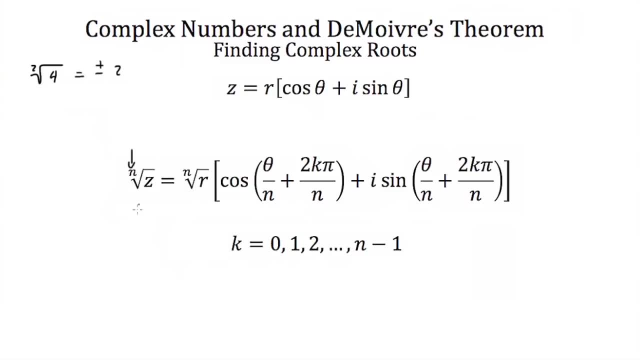 Our formula for doing this: if I have the nth root of Z, then we just take the nth root of our magnitude or our R value, and then it's multiplied by the cosine and we divide our theta by that N. But then to get the other solutions, 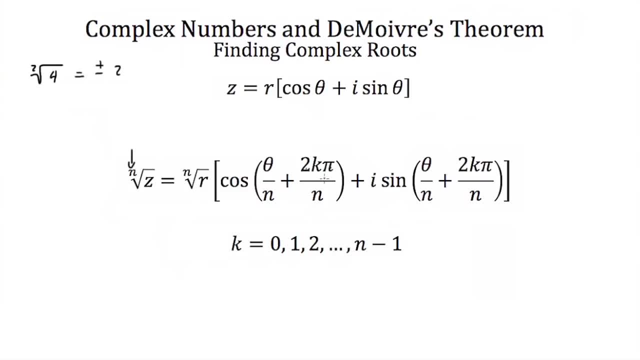 we add 2 pi over N and then multiplied by, we get the integral of k. k is this integer. Our first solution to our root k is equal to 0.. For the second solution of our root k would be equal to 1.. 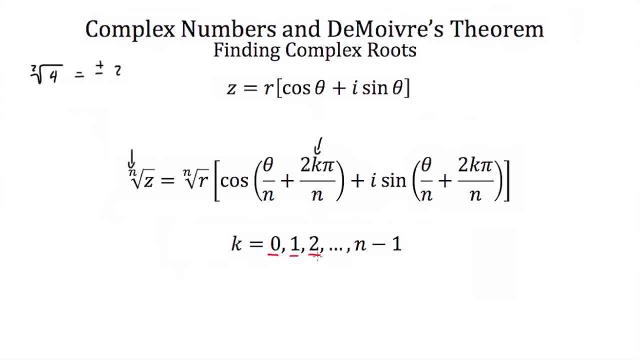 For the third solution, k would be equal to 2, and so on and so forth until we find all of the solutions for our root, All N of them. So if N is 4, there's four solutions. We do the same thing for the second solution. 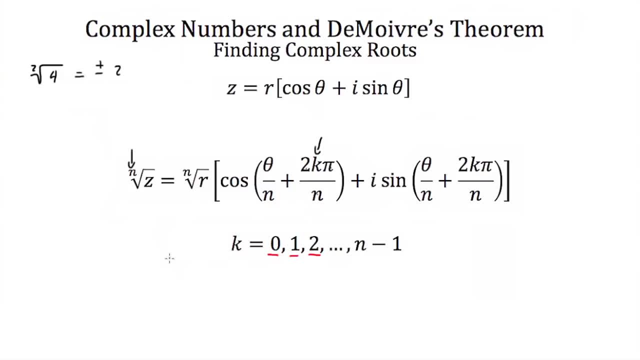 we do the same thing for the third solution and we do the same thing for the fourth solution. We do the same thing for the sine. take our original angle value and divide it by N, but then we add 2k pi over N. 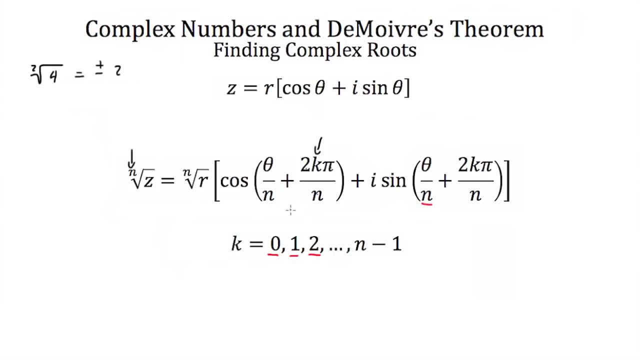 for each additional solution that we need Now. if you're not measuring in radians, realize that you don't need 2 pi here. Instead, you would be adding 360 times k over N. This 2 pi just represents one rotation around the pole. 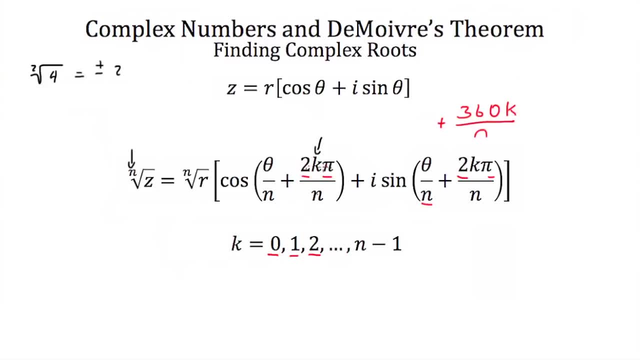 So if you're measuring in degrees, you would be adding 360 times k over N. This 2 pi just represents one rotation around the pole. So if you're measuring in degrees, you'd be adding 360 times k over N, Or else one full rotation around the pole would be 360.. 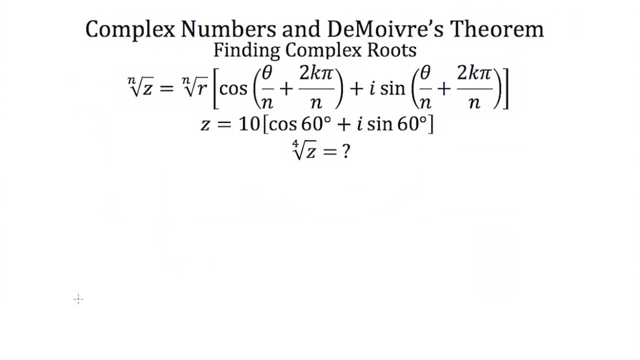 So let's try a practice problem. Let's take the fourth root of Z, where Z is equal to 10 cos plus i sin. So the fourth root of Z is equal to the fourth root of r, which is 10 times the cosine of theta, which is 60. 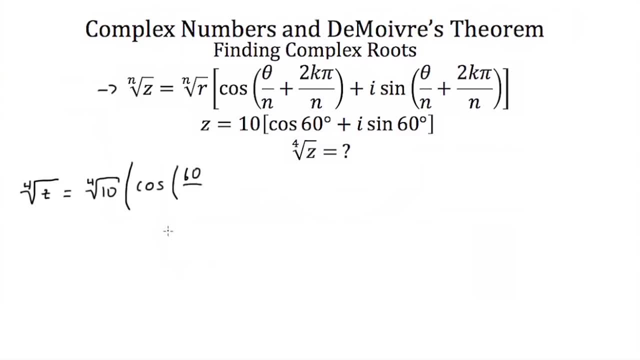 divided by n, which is 4 plus. now, I'm not going to use 2k, I'm going to use 360, because we're measuring our angle in degrees. so plus 360 times k, which, for our first solution, is 0 over n, which is 4 plus I times the sine of 60 over 4. 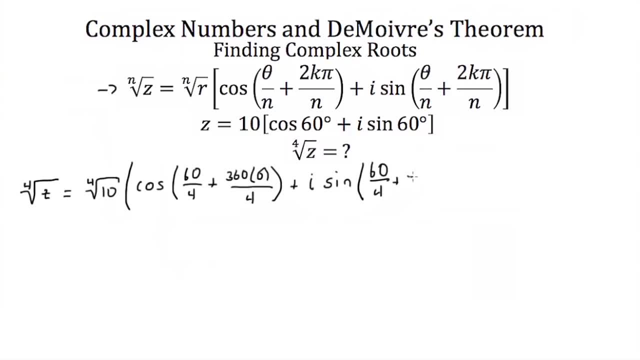 theta over n plus 360 times k, which in this time is 0, plus I times the sine of 60 over 4. theta over n plus 360 times k, which in this time is 0, plus I times the sine of 60 over 4, and this is our first solution, simplify it a. 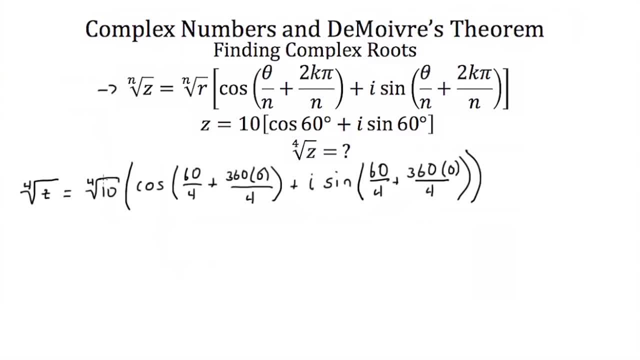 little bit. the fourth root of 10, that's 1.78, approximately 60 over 4, that's 15 degrees 360 times 0 is 0. 0 divided by 4 is still 0, so we have the cosine of 15. 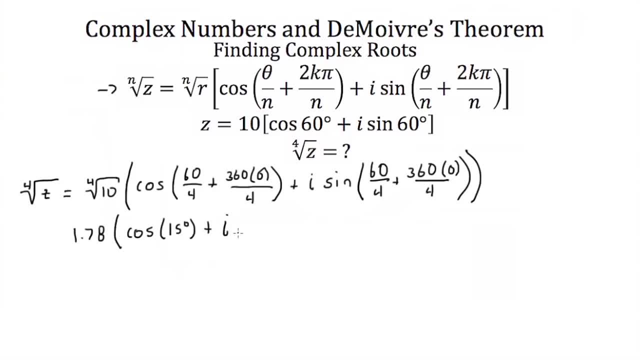 plus I times the sine of 15, and this is our first solution. now we're gonna end up with pretty much the same thing for our second solution, except our angle is going to be a little bit different. if we take this part or this part, they're the. 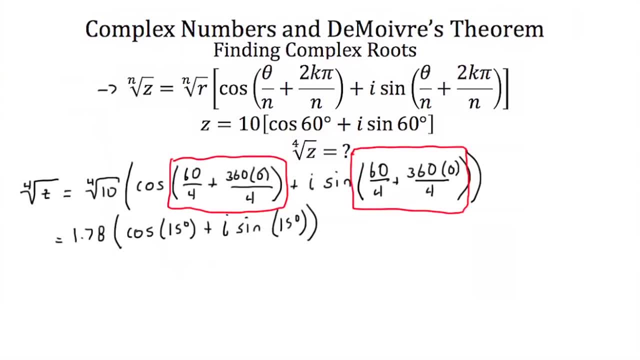 same for our next solution. we're going to solution. our K value goes up to 1.. So this is going to become 60 over 4, which is 15 degrees plus 360 times 1, this time over 4.. 360 times 1, divided by 4, is 90. so 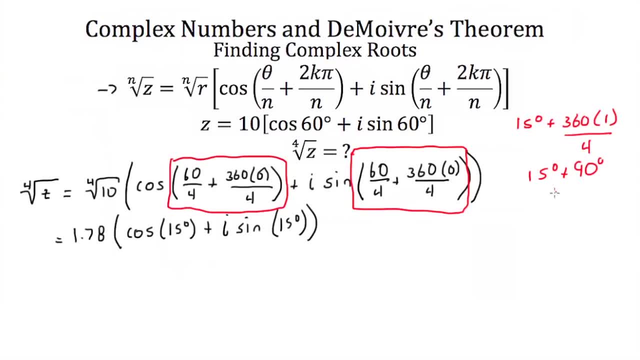 15 degrees plus 90 degrees, that's 105 degrees. So our second solution is 1.78 times the cosine of 105 degrees, plus I times the sine of 105 degrees. For our third solution, our K value goes up to 2.. So again, 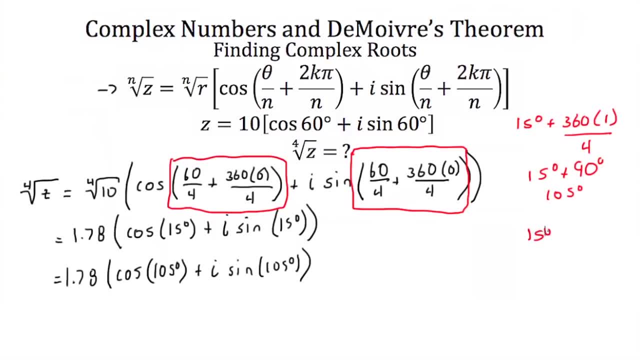 so we have 15 degrees 60 over 4, plus 360, this time times 2 over 4.. This is equal to 180. so I have 15 plus 180, which is equal to 195.. So my third solution for this root is 1.78. 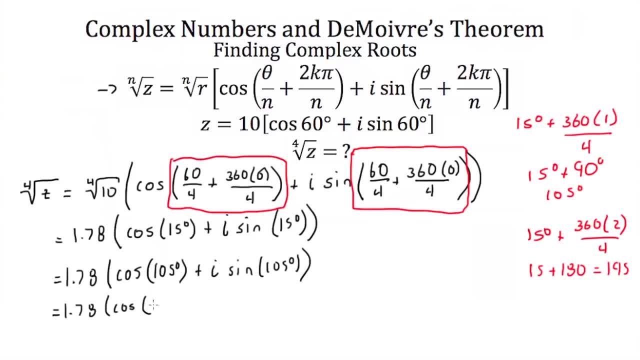 times the cosine of 105 degrees. So our third solution for this root is 1.78 times the cosine of 105 degrees. So our third solution for this root is 1.78 times the cosine of 105 degrees. So our third solution for this root is 1.78 times the cosine of 105 degrees. 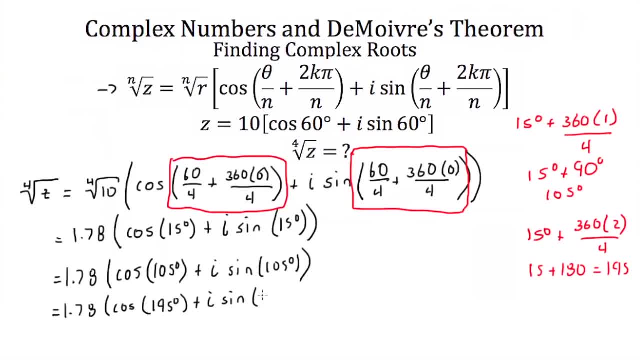 So we have 25 Crepes for the Pre terrace. Mach Growth 436. I'm going to break it down for now. this is 1.87I times the sine of 얘 소�. undergo una X tomar 100, 1. Mental. 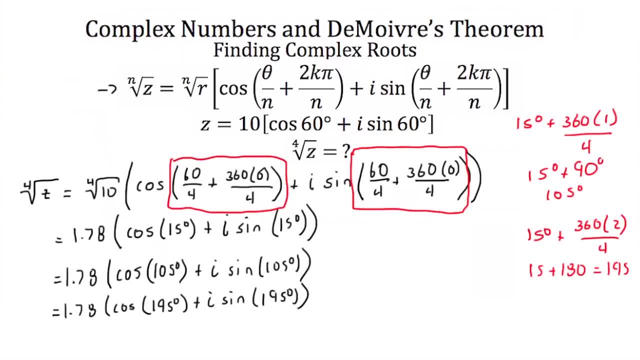 1 more solution to go for my 40, and divided by 4, is 3.5 times the sine of 195 degrees, plus I times the sine of 195 degrees. One more solution to go for my 40, and divided by 4, is 3.5 times the sine of 125 degrees For my 41. fourth, I go up. 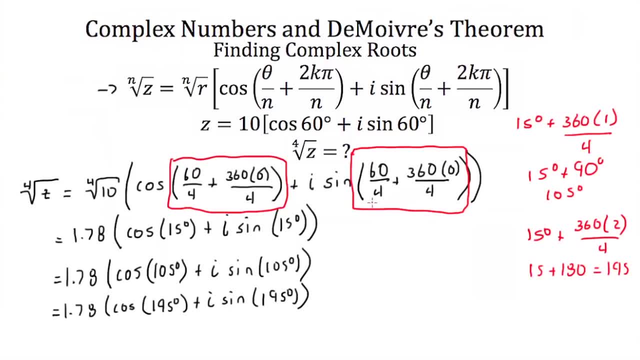 5 degrees. So 60 over 4 is 15 again. so 60 over 4 is 15 again, plus 360 times 3, this time over 4.. And divided by 4 is 270 times 3.5 is 270. so 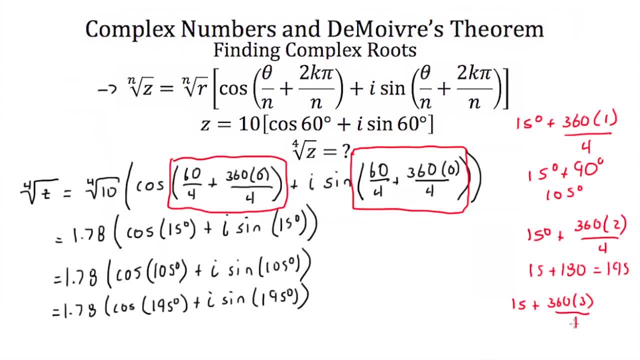 we come triple 60 times 3, this time over 4.. This culminates when we take shim. be ready. So our second solution for this root of 15 degrees times 3 and divided by 4 is 270.. So 15 plus 270 is 285.. So my fourth solution is 1.78.